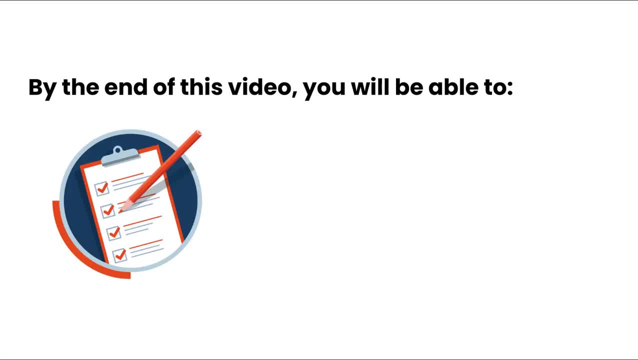 In this video we're going to take a look at how to charge objects by two different methods, called contact and induction. So by the end of this video, you'll be able to: 1- explain the use of an electroscope, 2- describe how different materials can be charged by contact, and. 3- describe how. 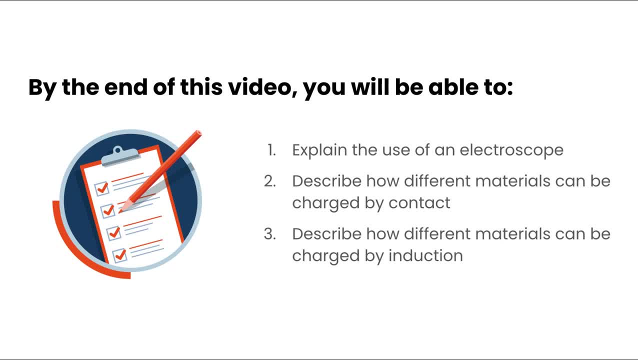 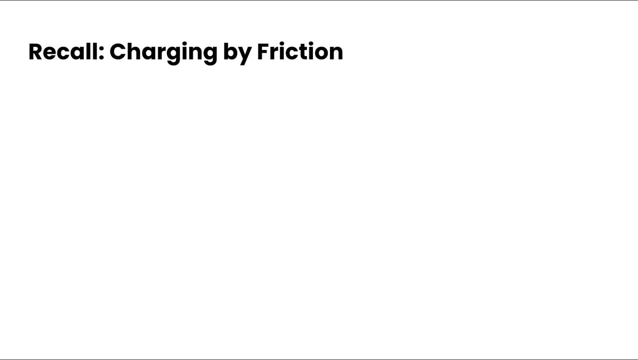 different materials can be charged by induction. So let's just jump right into it Now. we first kind of want to start by remembering what does it mean to charge an object, And one of the ways that we've done that so far is charging by friction. So, charging by friction. 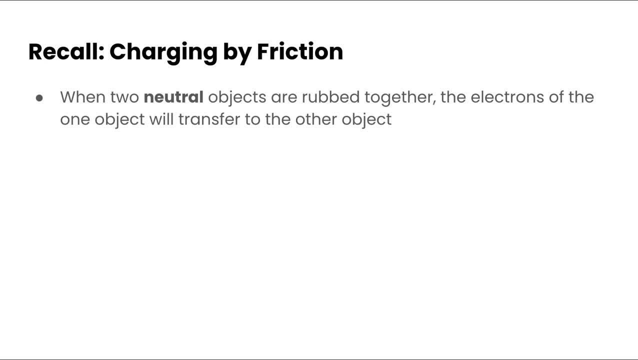 happens when two neutral objects are rubbed together and the electrons from one object will transfer to the other. So if you remember from a previous lesson that if we took an uncharged cloth and an uncharged plastic rod and rub them together, the charge or the electrons would transfer from the rod, 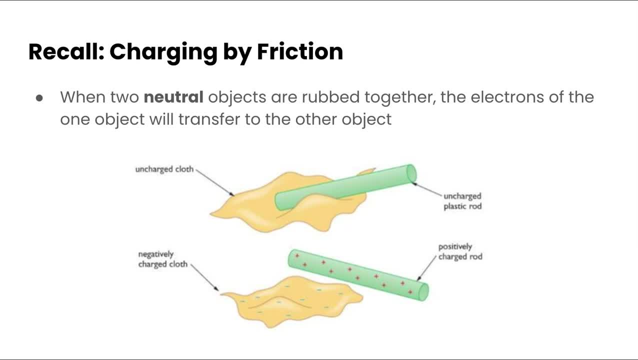 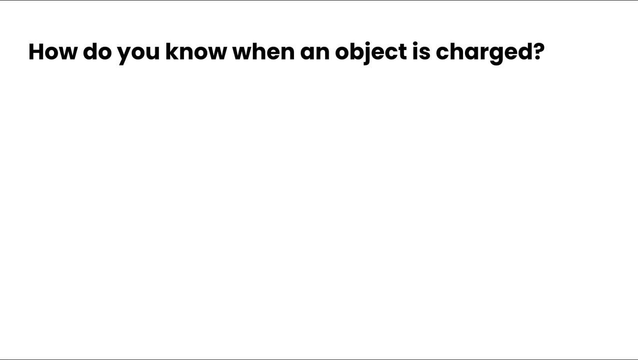 onto the cloth here. So the cloth would take a negative charge and the rod would take a positive charge. So that is charging by friction. Now, how do you know when an object is charged? Well, instead of testing whether an object just sticks to something else, you can use an instrument called 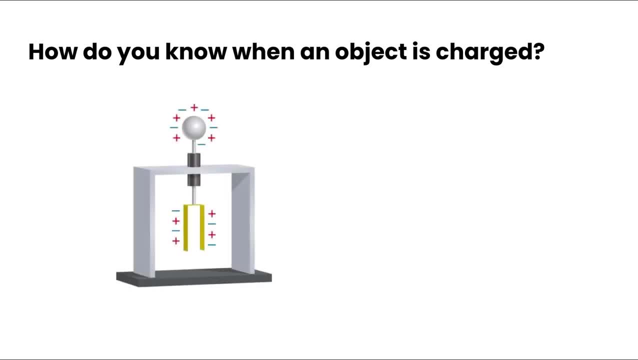 an electroscope. So an electroscope looks like this. This is a metal leaf electroscope. It has a metal ball at the top- here It's connected by metal down to the inside part- here- And then it has two leaves, And these leaves are normally made up of gold. 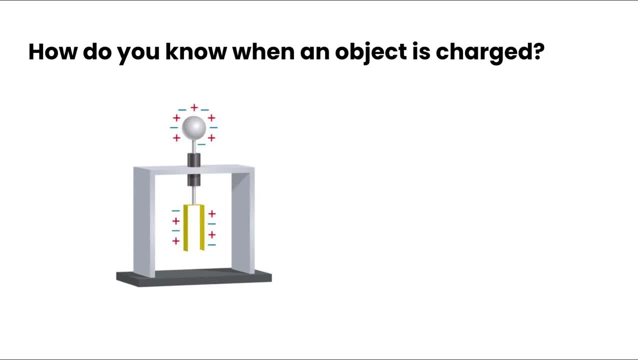 sometimes other metals. But what you can do is then use this object or this apparatus to to see if something has a static charge or not. And so what you do is you bring an object close to this metal ball or you can touch the metal ball And, for example, if we brought a rod close by that, 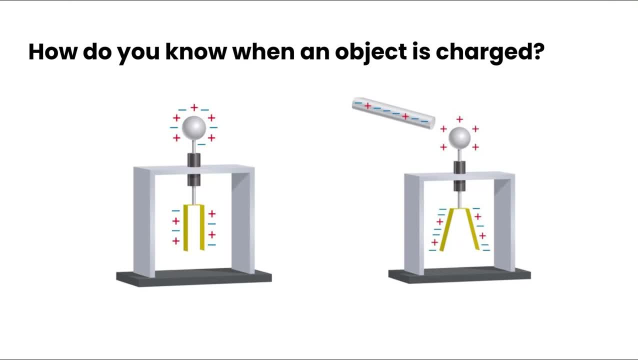 had a negative charge, then what it's going to do by induction is push all those negative charges in the metal ball piece here down into the leaves, And so those negative charges are going to distribute themselves evenly between the two leaves And because of the law of repulsion, 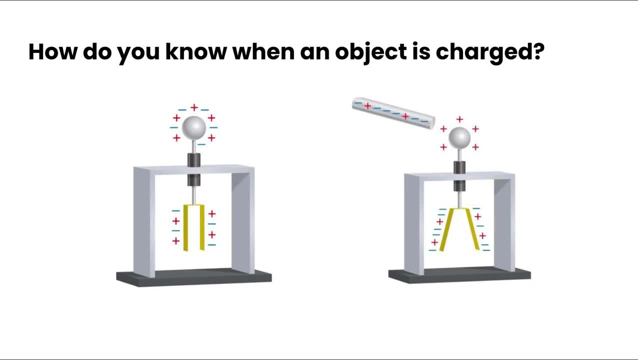 they are going to repel each other and move apart. Now, if we pulled this rod away, the electrons would redistribute themselves again, no longer being repelled, and the leaves are going to drop down, So this is a great instrument to see like: do we have a charge? 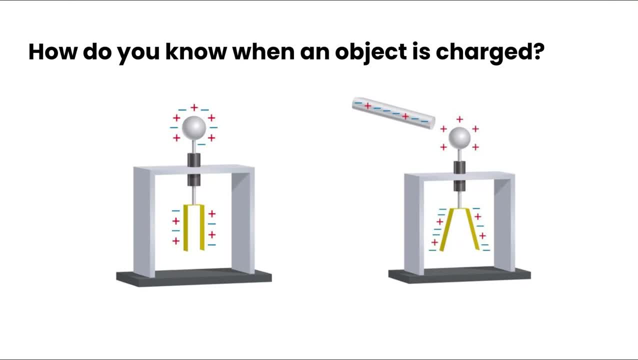 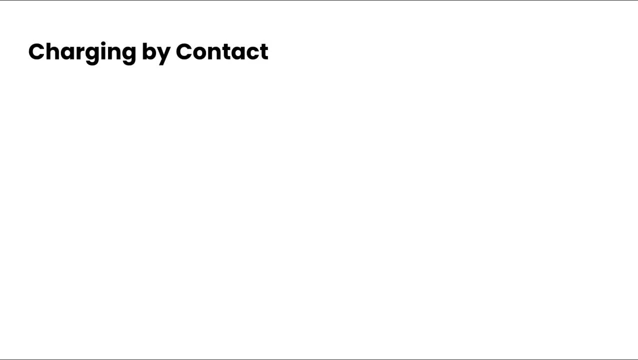 And we can tell just by doing a very, very easy experiment. Now, let's first start about with charging by contact. So what is this? Well, you can charge a neutral object by contact when you touch it with a charged object. And when you touch it with a charged object, the electrons. 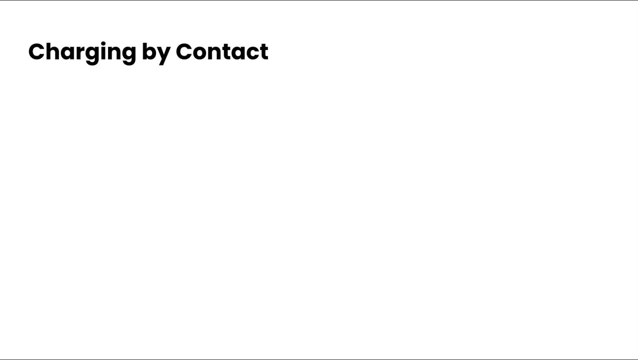 will transfer from the charged object to the neutral object that it touches. So if we take a metal ball, for example, here's our electroscope, a very simplified version of our electroscope. we see that all of our charges are evenly distributed across it and the metal leaves. 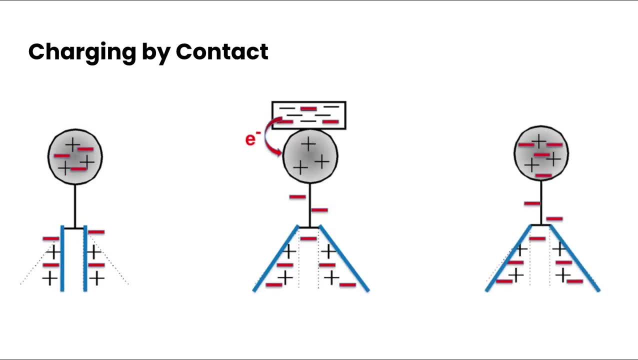 are down Now. if we were to bring a negatively charged rod close and then touch the metal ball at the top, electrons will transfer from the rod to the ball, and then they will get repelled down into the leaves, And so the two metal leaves will move apart and be repelled from each other. 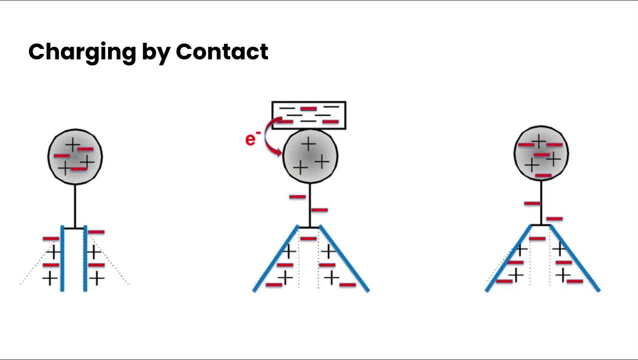 Now, because we have transfer of electrons here. if you take the negatively charged rod away, those leaves stay open because we have now gained more negative charge. So that is going to make this once neutral electroscope now now also have an overall negative charge because we touched it with an overall negative object. 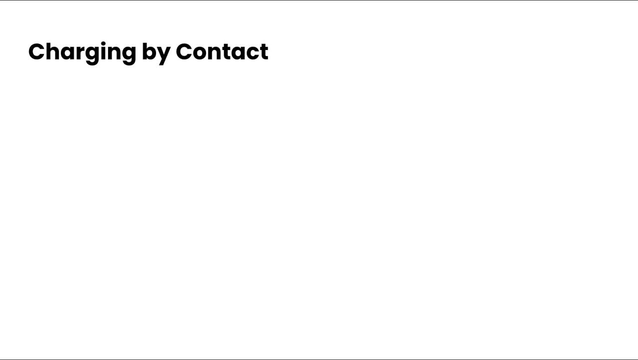 You could do the same and do the same sort of reasoning if we touch a positively charged object to a neutral electroscope. So here's our neutral electroscope again. If we bring in a positively charged rod now, the electrons are going to transfer from the electroscope into the rod. 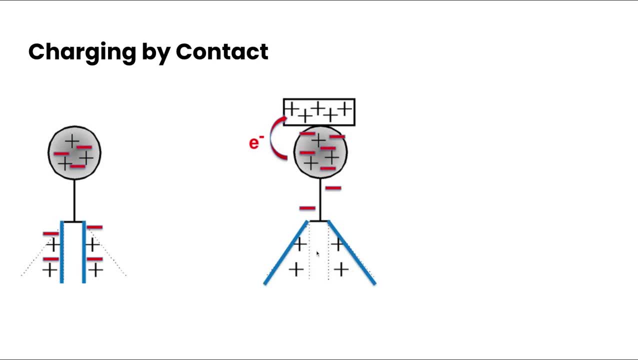 Again pushing these leaves apart, because now we have positive charges distributed amongst both, And then when we remove the rod, those leaves remain open and the neutral object is now positively charged overall. Charging by induction is a little bit different, So we kind of touched on this a. 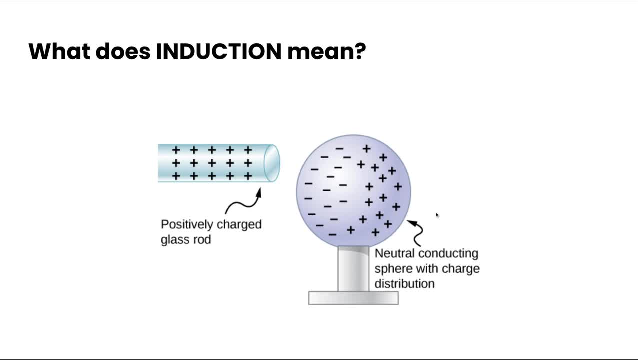 little bit earlier in this video. but what does induction mean? Well, induction really uses the laws of attraction and repulsion to rearrange the electrons in an object, to change the charge on that surface, on the object. So, for example, if we were to bring a positively charged rod, 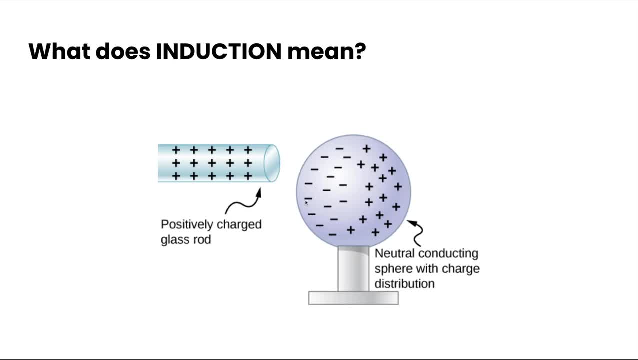 close to the ball of an electroscope but don't touch it then, because we have a positive charge here. it's going to rearrange the electrons. So the electrons are close. they're not going to change the charge on the ball of an electroscope. So what we're going to do is: 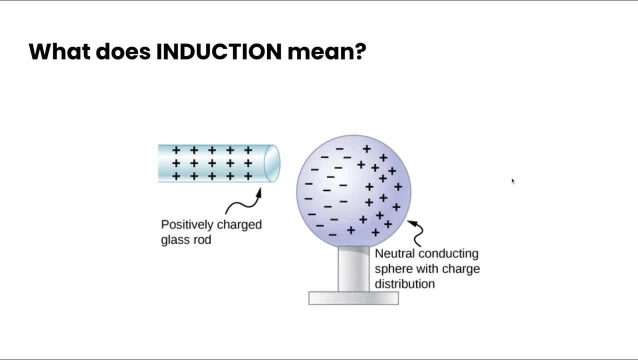 we're going to move the rod closer to the positive charge and then all the positive charges are further away. So in this example, the positively charged rod is we say, is inducing a charge on the sphere because it charges the sphere without touching it. But if we were to remove this rod? 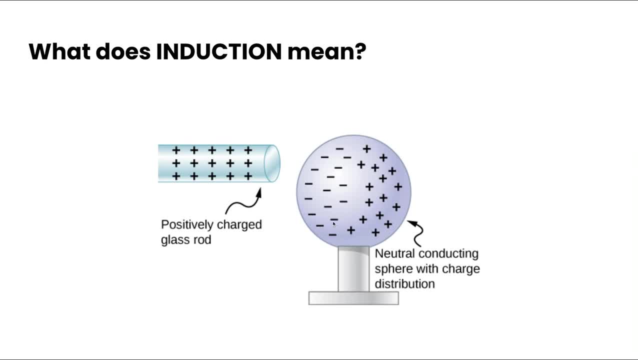 the distribution of these charges would return back to normal and it would go back to a neutral charge. Now, if we were to remove this rod, it would return back to normal and it would go back to a neutral charge. But if we wanted to make something permanently charged by induction, we need a concept called 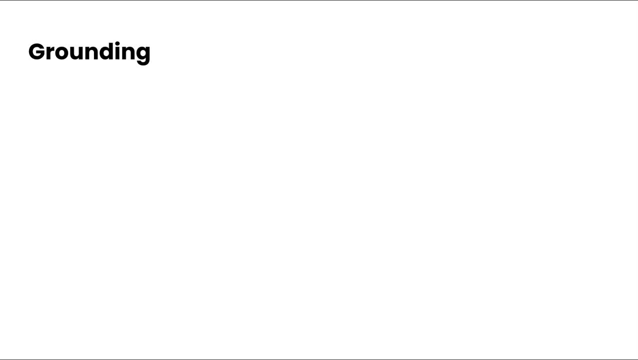 grounding. So what is grounding? Well, when we connect a charged object to the Earth, that's what we call grounding, And the reason that we use this, or the purpose of this, is that the ground itself on Earth can absorb extremely high amounts of electrons while still remaining. 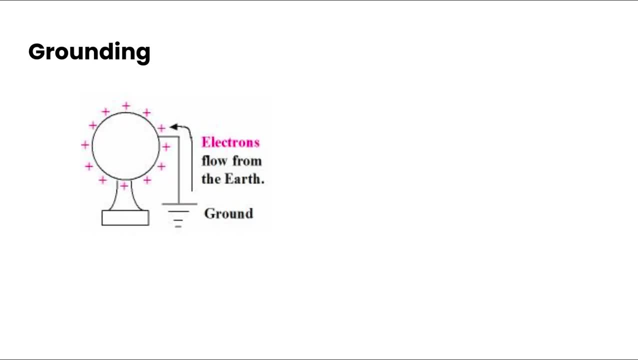 neutral, And that's because the ground itself on Earth can absorb extremely high amounts of electrons while still remaining neutral. And that's because the ground itself on Earth can absorb extremely high amounts of electrons while still remaining neutral, And so it can either accept electrons or donate electrons, depending on 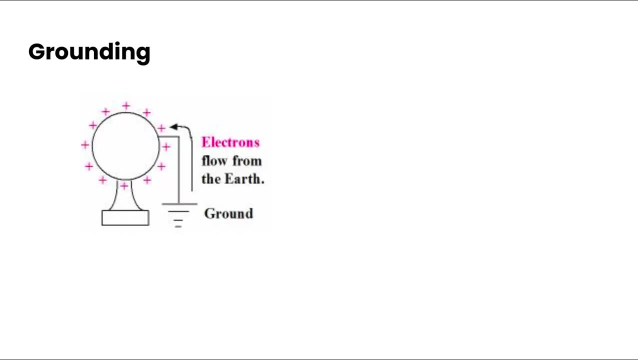 the overall charge of the object that is touching the Earth. And so, for example, if we were to take a positively charged electroscope and we grounded it, so connected it to the ground, somehow electrons will flow up into it, reverting it back to a neutral charge. 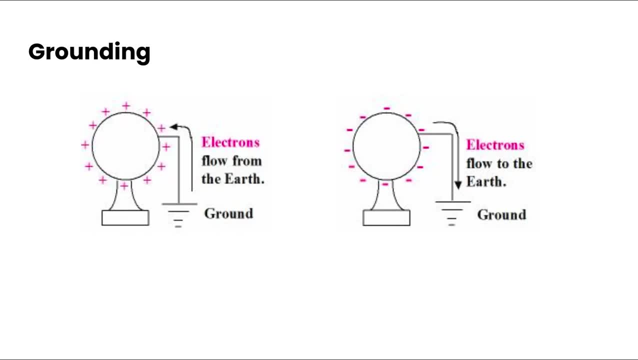 Now, if we did the opposite, so we took a negatively charged electrosphere and grounded it, the electrons would flow back into the Earth again, restoring that neutral charge on the electroscope. Now why is this important? for induction? Well, we can actually take an induction. 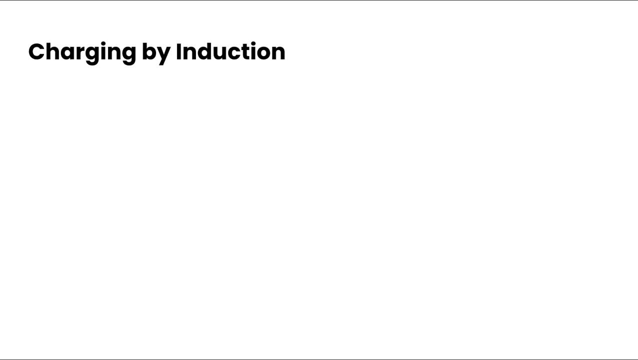 and if we ground it we can create a positive, a permanent charge rather than just an induced charge. So let's kind of walk through the steps here. We first: if we bring this positively charged rod close to an electroscope, we get that rearrangement of electrons. okay, Now 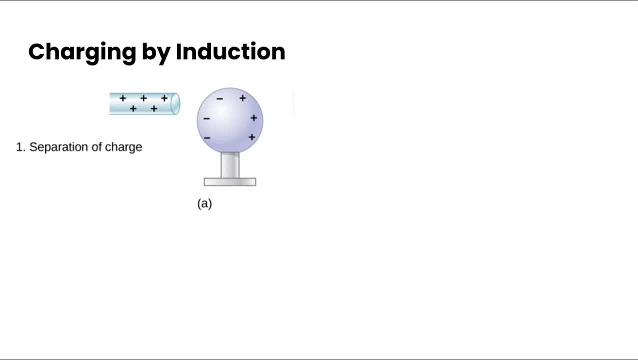 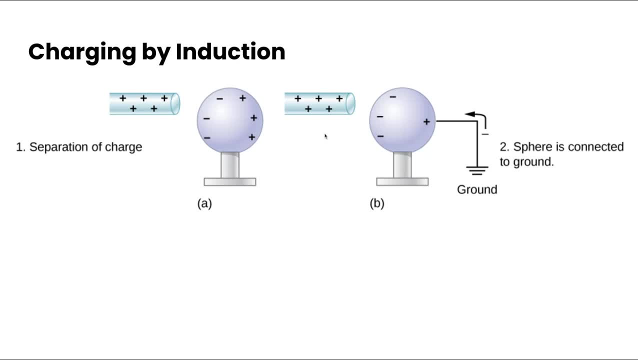 if, instead, as we held, that positively charged rod close to our sphere, if, instead, as we held that positively charged rod close to our sphere, then, because we've got this rearrangement of electrons here, we've got a more sort of positive end. 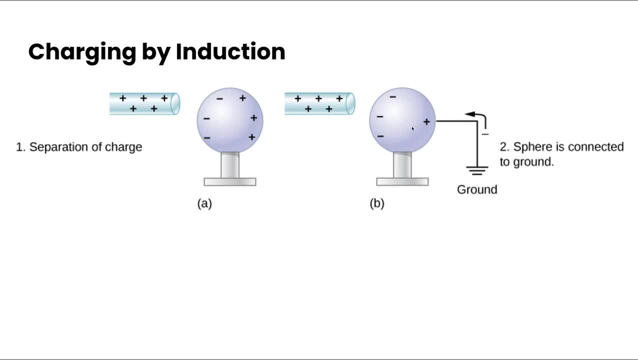 and so electrons are going to come up into the sphere to help balance this positive charge that is nearby. Now then if we disconnect the sphere from the ground but we still hold that positive charge there and then finally remove the positive charge, then, because we've got this rearrangement of electrons here, we've got a more sort of positive charge there and then finally remove the positive charge that is nearby. 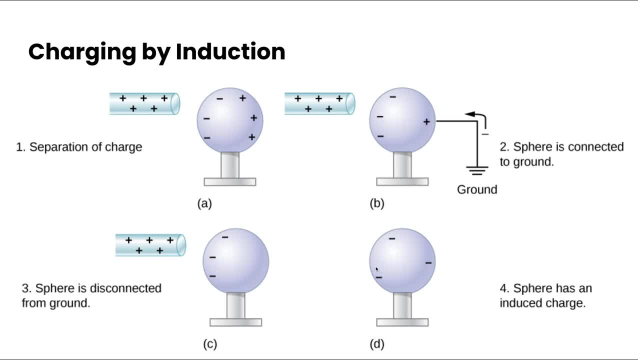 The sphere overall is going to keep an induced negative charge. So this is one way that we can go about and cycle through to get a negative charge without ever touching it, and by only touching it to the ground. All right, so we went over charging by contact, charging by induction. 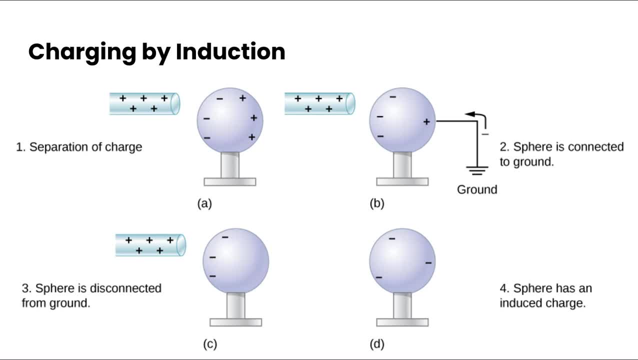 and what grounding is. That's it for this video. Let's move on to our next task.